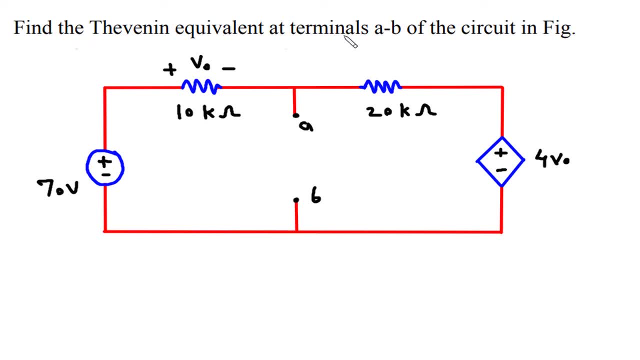 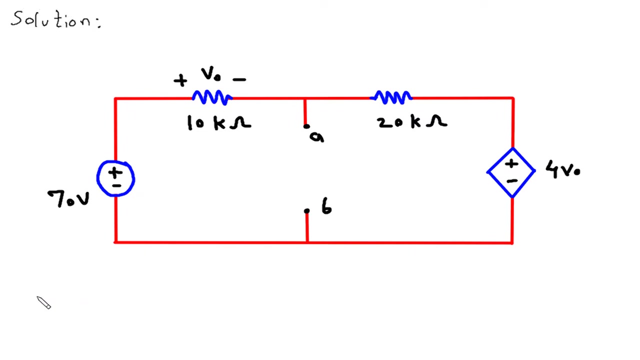 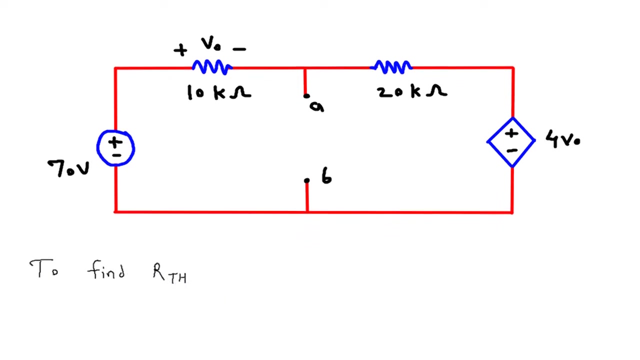 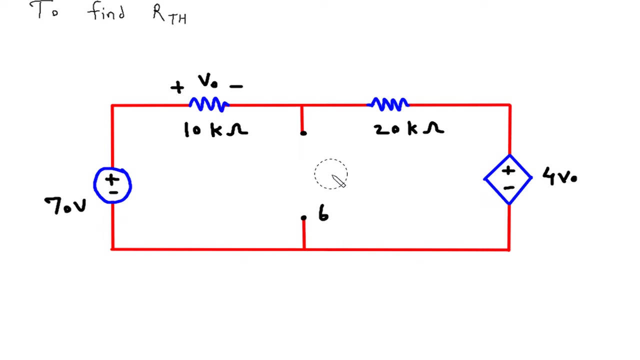 Find the Thevenin equivalent at terminals A, B of the circuit in figure. We have to find the Thevenin equivalent of this circuit solution: First we will redraw the circuit Now. first we will find Rth. So to find Rt we will consider. to find Rth We will assume a one volt voltage source. 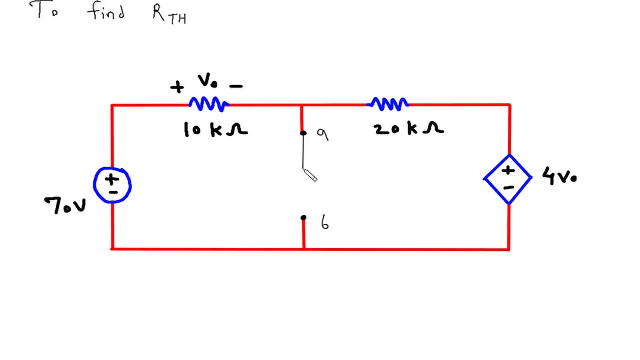 This is terminal A, This is terminal B and let's say this is one volt voltage source. This is positive and this is negative. This is one volt. This will be short-circuited to find Rth. Now, this is a dependent source. That's why we have considered this one volt. 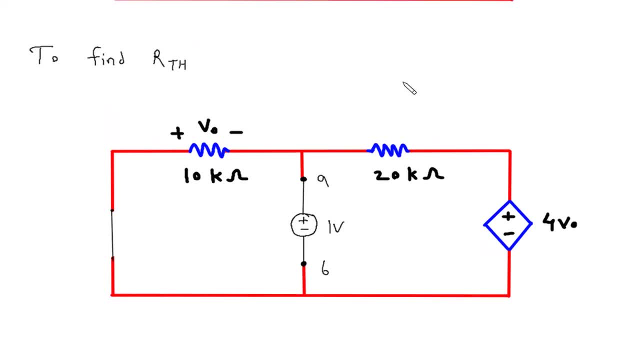 voltage source to find Rth. Now, Rth is equal to. Rth is equal to voltage, which is one volt divided by current. Now we have to find this current. let's say this current is this current is Io. 1 by Io is equal to Rth. Now we have to find this Io. Now, let's assume this is: 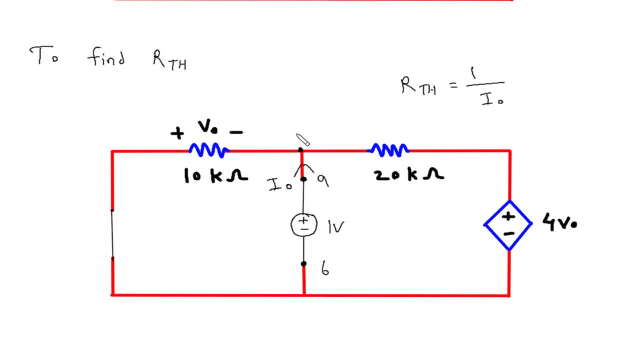 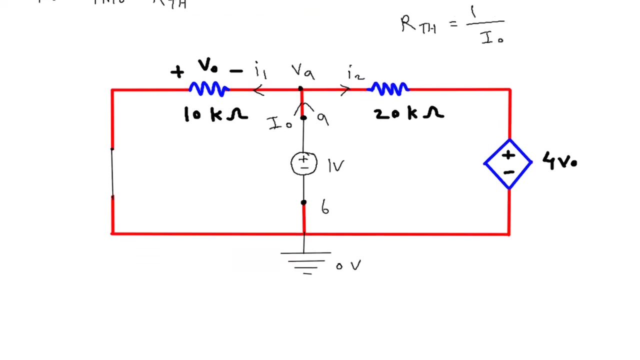 node. this is node Vo or Va. this is ground node with zero voltage. This is current. let's say, this is current I1. And this is current I2.. Now we will apply KCL at node VA. So summation of all the entering current. entering current is IO. 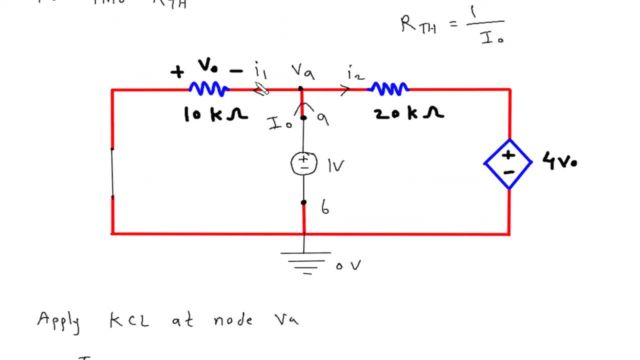 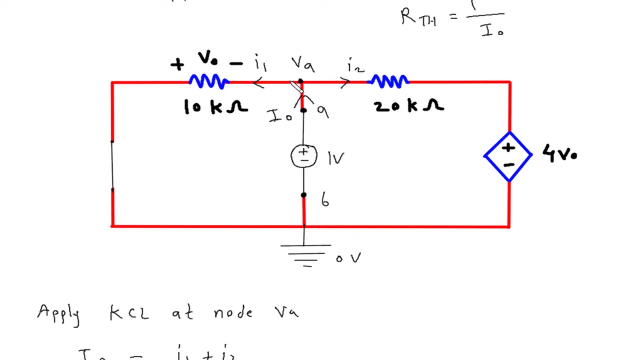 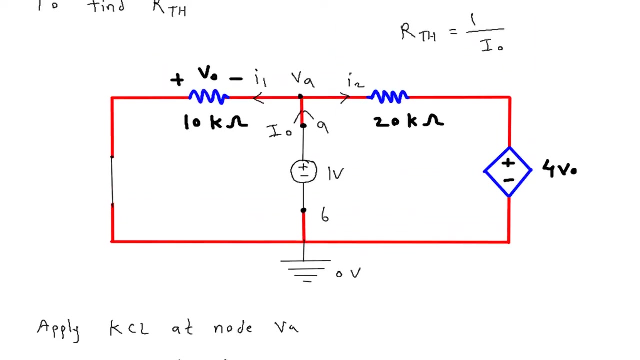 And leaving current at this node is I1 plus I2.. Now IO is 1 minus VA, or directly we can write IO is equal to. we will write IO as it is, Then I1.. I1 is VA minus 0.. VA minus 0 by 2.. 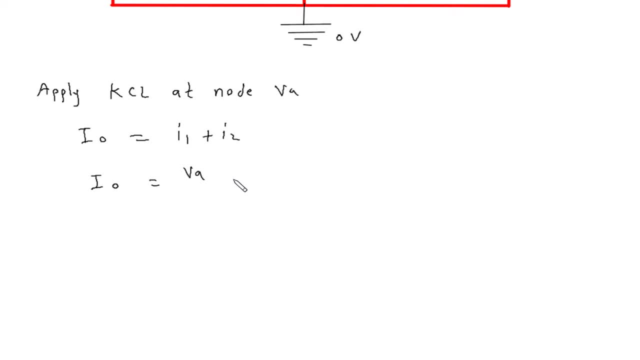 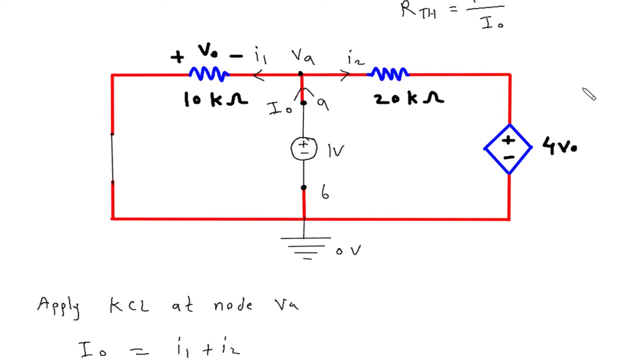 That is 10 Kilo ohm. VA minus 0 by 10 Kilo ohm, that is 10000 plus I2.. Now I2 is VA minus 4VO. VA minus 4VO divided by 20 Kilo ohm. 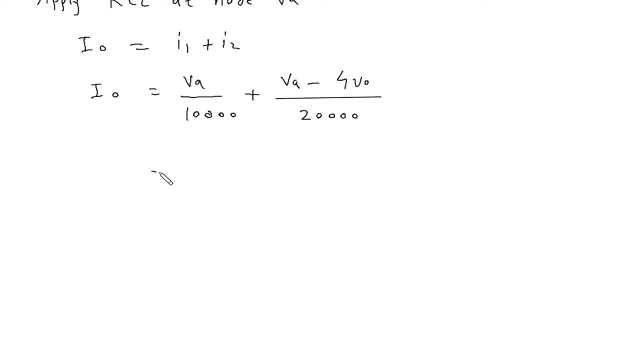 So 20000.. Now this will be VA divided by 10000 plus VA divided by 20000 minus 4 by 2000,. 20000 into this VO. Now this VO is VO is 10000 minus 10000 because the polarity is opposite. so minus 10000 into I1.. 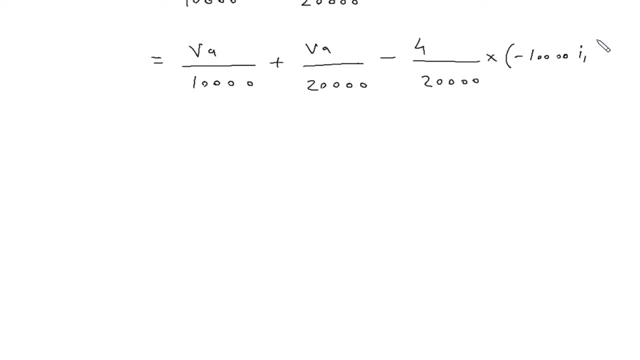 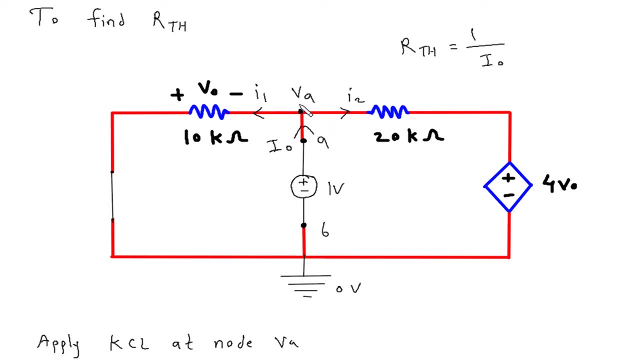 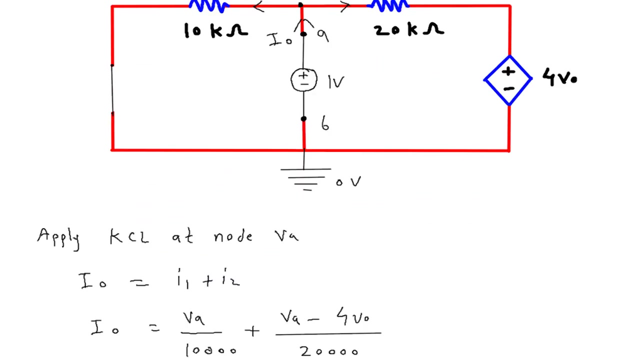 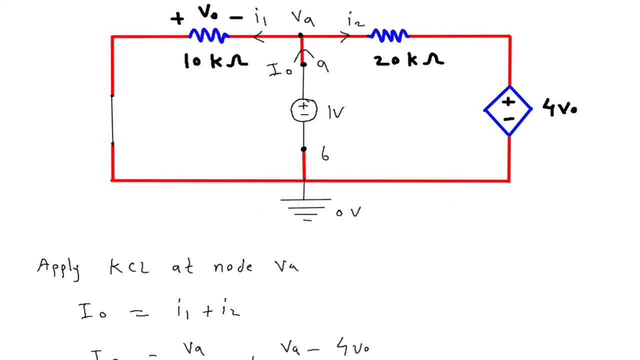 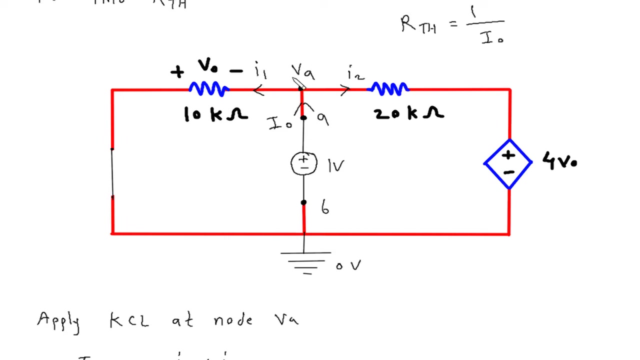 Minus 10000 into I1. And I1 is VA. VA minus VA minus 0 by 10000.. Or directly we can write VO is equal to minus VA. From the polarity, we can write VO is equal to minus VA. 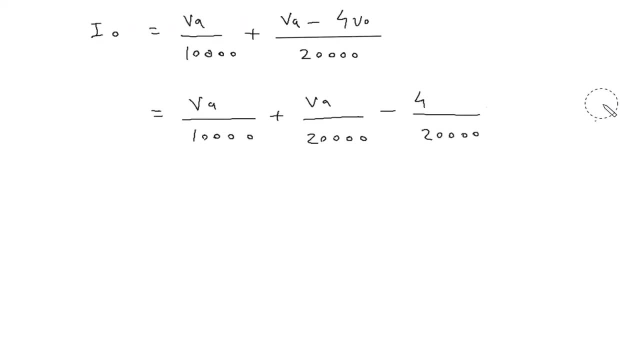 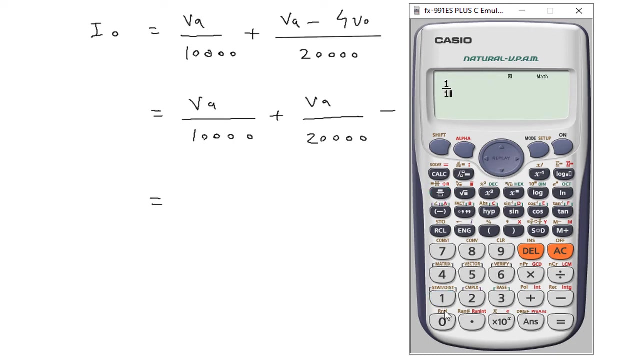 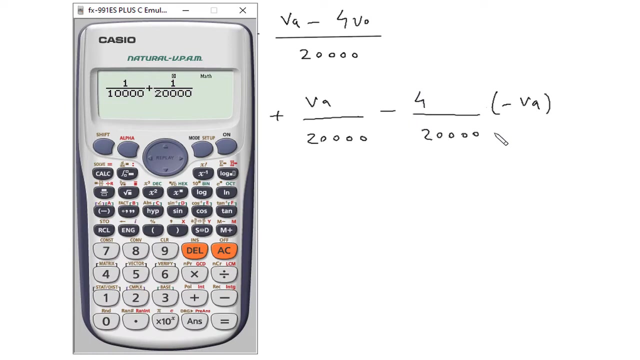 So this will be directly minus VA. Now this will be 1 by 10000. So this will be 1 by 10000.. 1 divided by 10000, then plus 1 divided by 20000. Then this will be minus minus plus, so plus 4 divided by 20000. 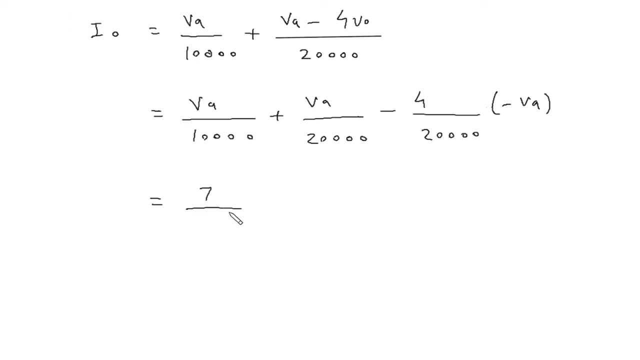 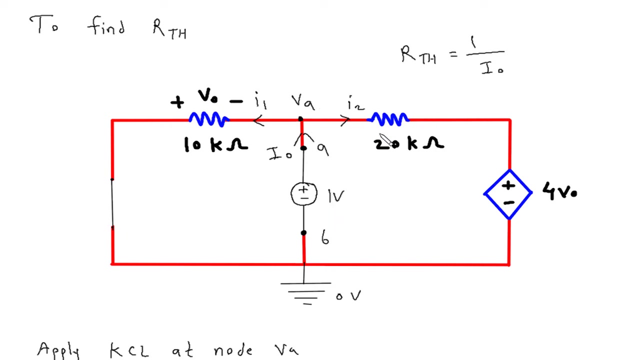 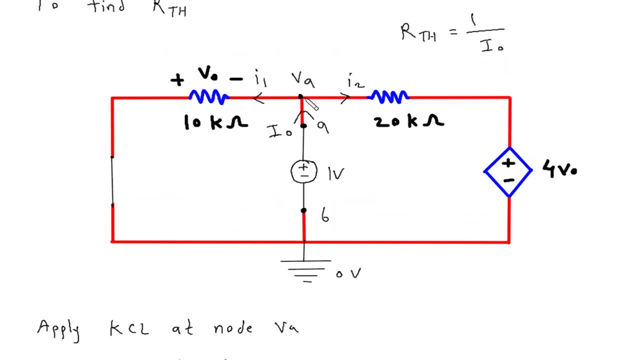 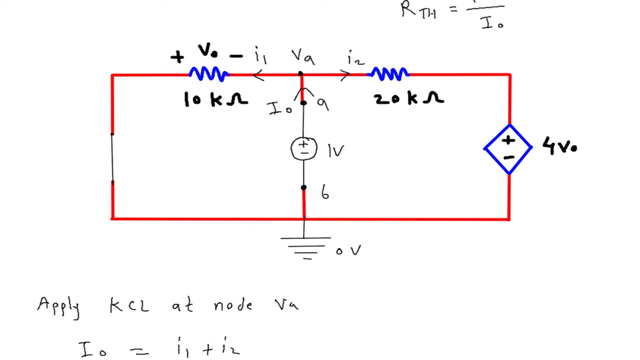 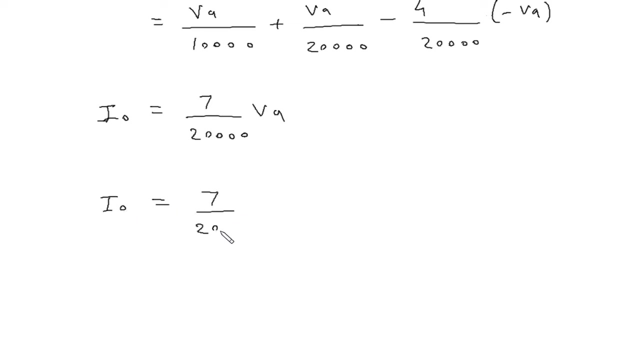 So this is 7 divided by 20000.. VA: this is the value of IO. Now VA is equal to. VA is equal to directly. We can say that VA is equal to 1 volt because it is connected to ground. So this will be: IO is equal to 7 by 20000.. 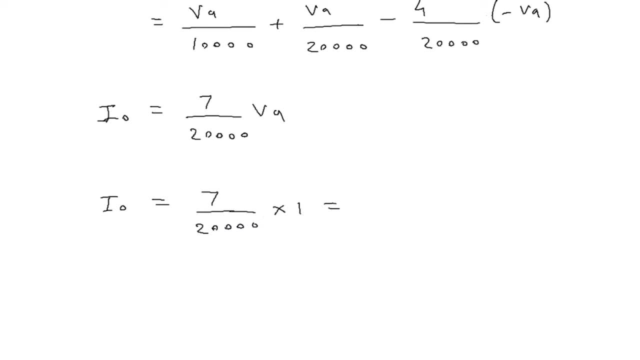 Into 1 is equal to 3.5. into 10, raise to minus 4. ampere is the value of IO. Now from this we can find the value of RTH, RTH. RTH is equal to 1 by IO. 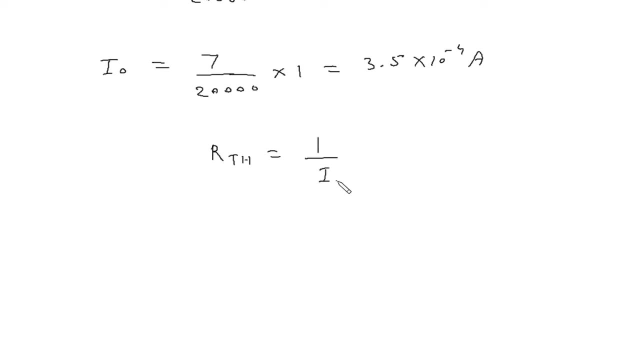 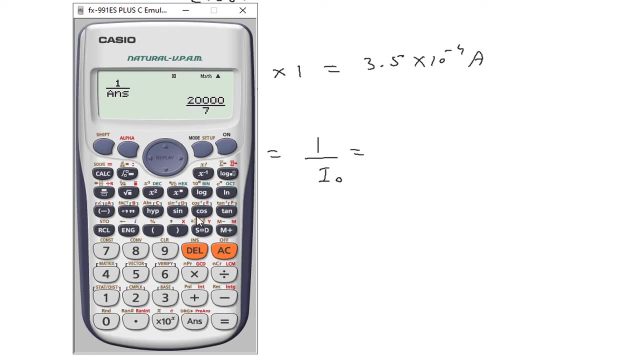 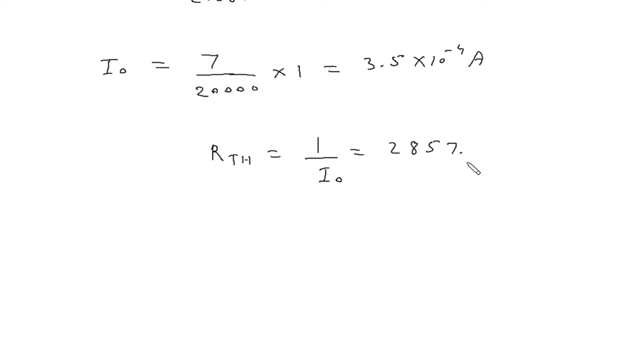 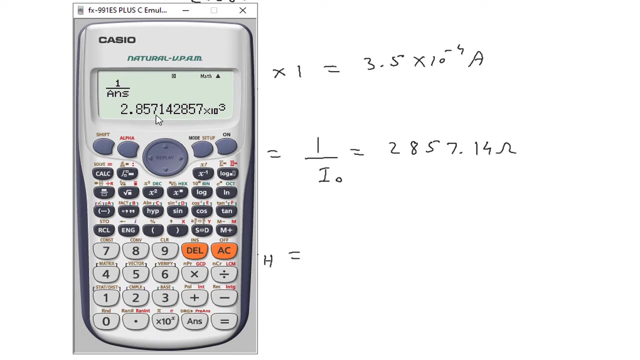 RTH is equal to 1 by IO, So this will be 1 by 2857.14 ohm is the value of RTH? Or RTH is equal to 2.857 kilo ohm. This is the value of RTH. 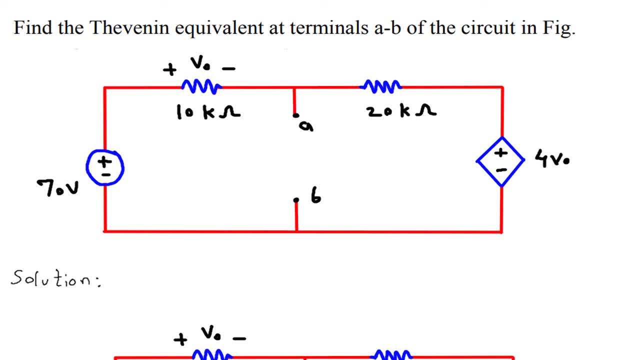 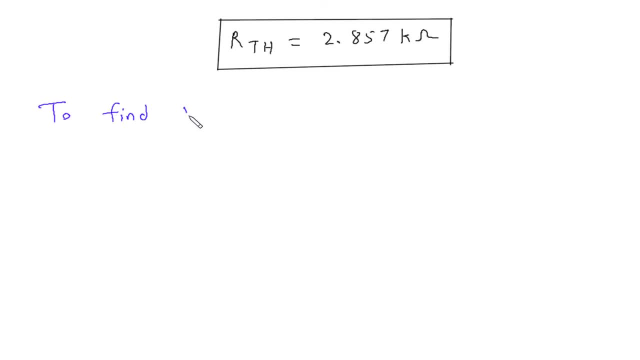 Next we have to find VTH. So to find VTH, To find VTH, This will be VTH. Now, to find VTH, We will apply, Let's say, this is current I1 and this is current I2.. And this is node VTH. 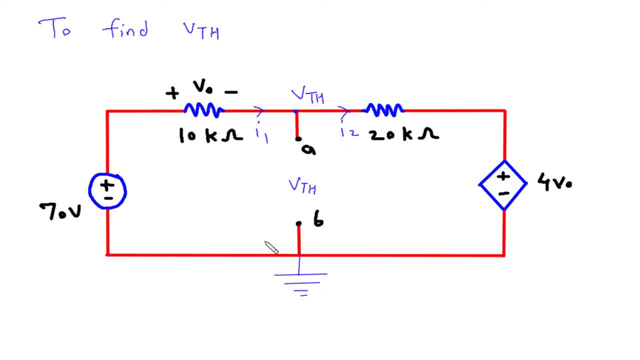 This is ground. Now we will apply. Apply KCL. Apply KCL at node VTH. So this will be summation of all the entering current. I1 is equal to summation of all the leaving current, So I2.. I1 is equal to I2.. 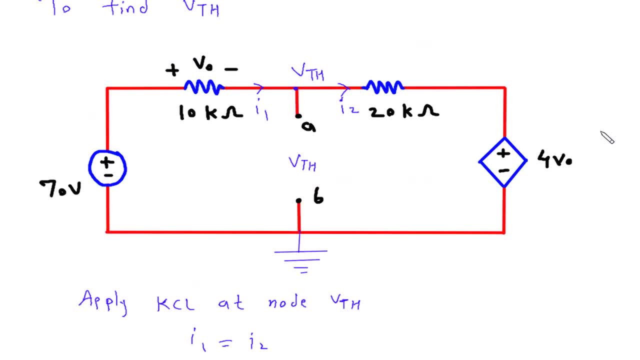 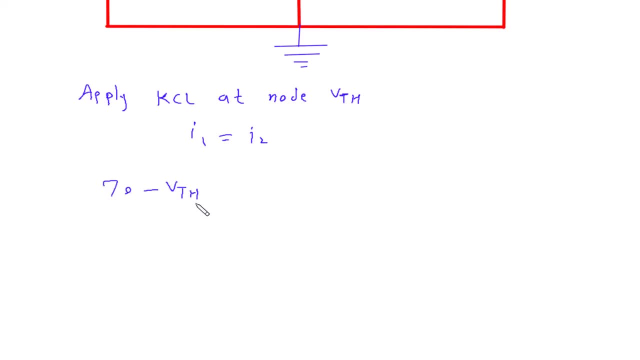 Now I1 is 70.. 70 minus VTH by 10 kilo ohm. 70 minus VTH by 10 kilo ohm is equal to I2.. I2 is VTH minus VTH minus 4VO. 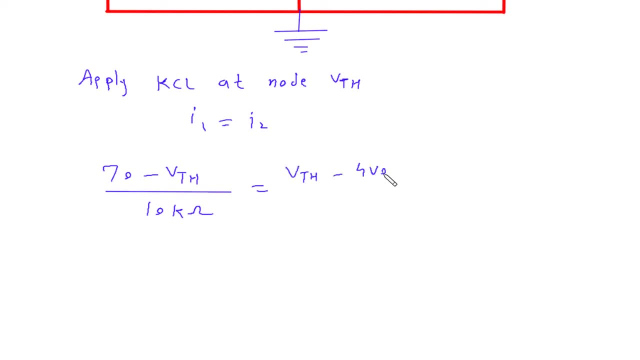 VTH minus 4VO divided by 20 kilo ohm- 20 kilo ohm, So this will be 70 by 10,000.. This is 10,000.. Minus VTH by 10,000.. 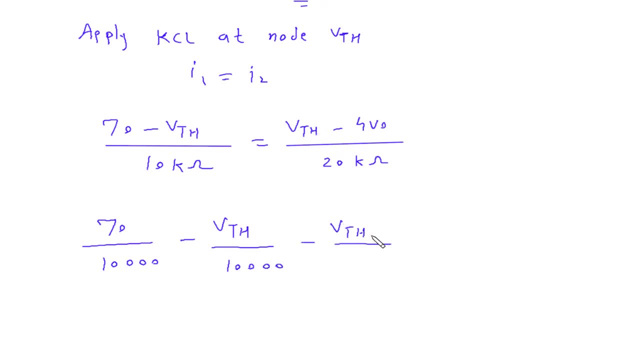 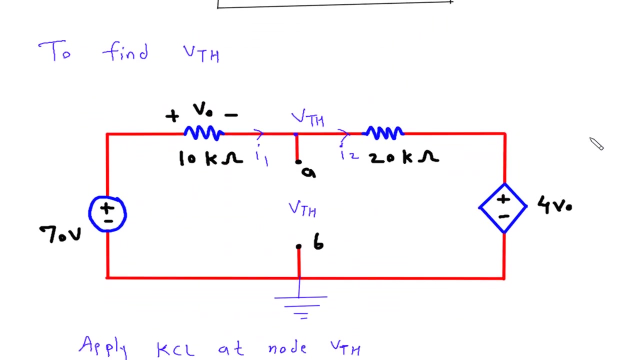 Then minus VTH by 20,000.. Then this will be plus 4 by 20,000 into VO. Now, in place of VO, we can write This: VO is equal to: VO is equal to 70 minus VTH. VO is equal to 70 minus VTH. 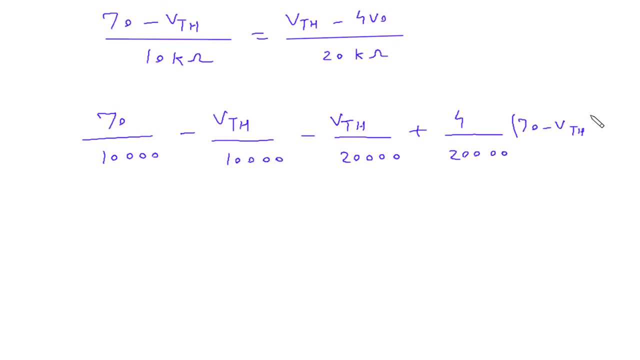 So 70 minus VTH Is equal to 0.. Now this will be 70 by 10,000.. So this will be 7 by 1000.. 7 by 1000 minus VTH, by Or directly, we will solve this. 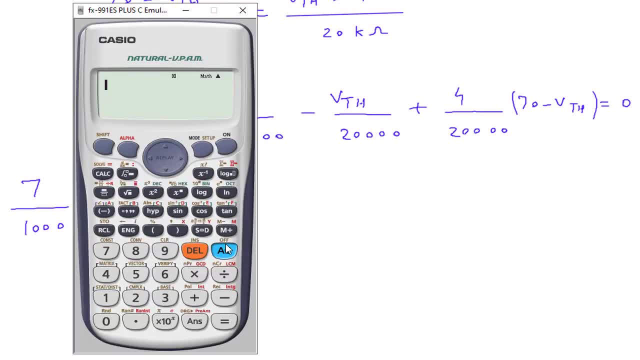 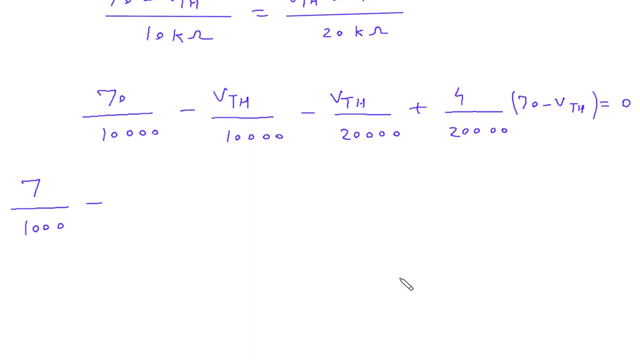 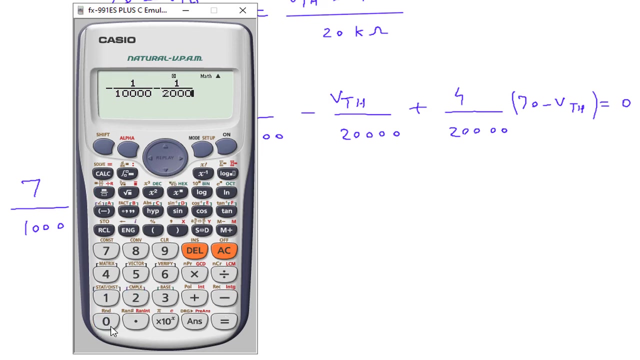 So this will be: Minus 1 by Minus 1 by 10,000.. Minus 1 by 10,000.. Then minus 1 by 20,000.. Minus 1 by 20,000.. 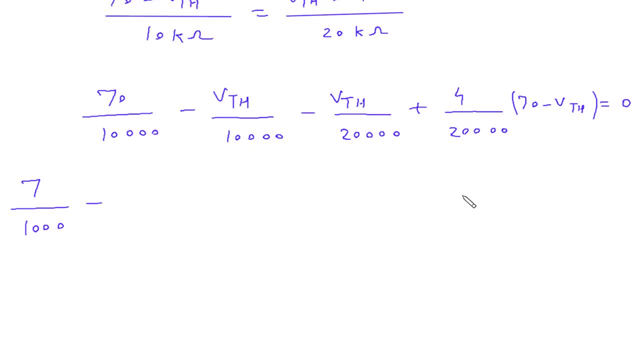 So minus 3 by 20,000.. Minus 3 by 20,000.. Minus 3 by 20,000.. VTH Plus 4 into 70.. 4 into 70 by 20,000.. 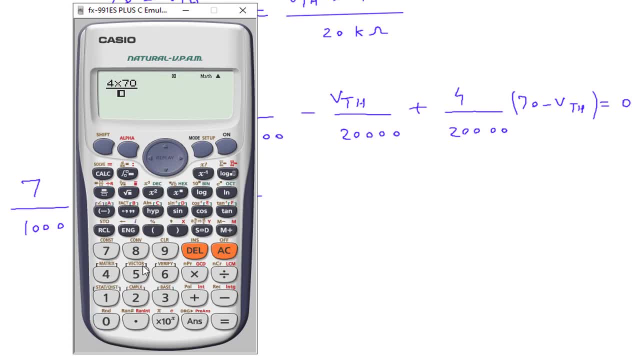 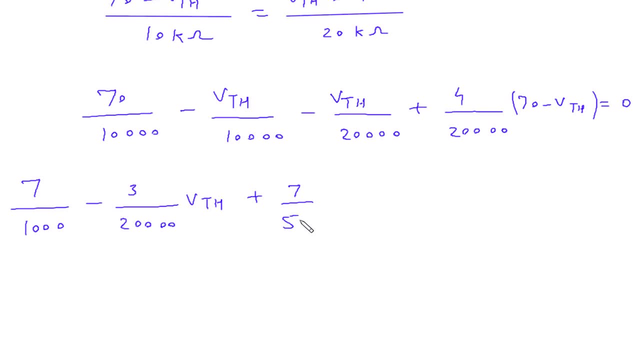 So 4 into 70.. Divided by 20,000.. 7 by 500.. 7 by 500.. Then minus 4 by 20,000.. 4 by 20,000.. 4 by 20,000.. 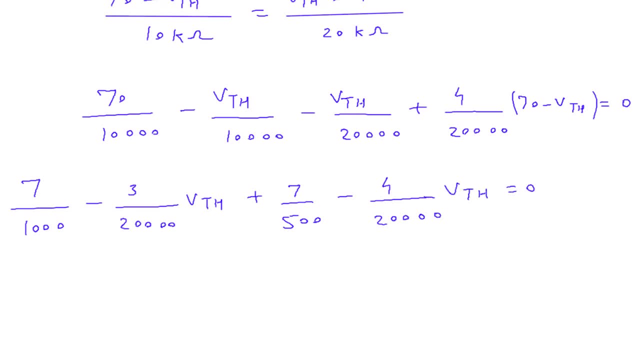 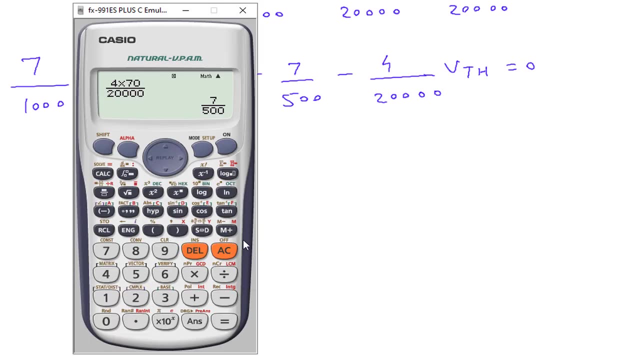 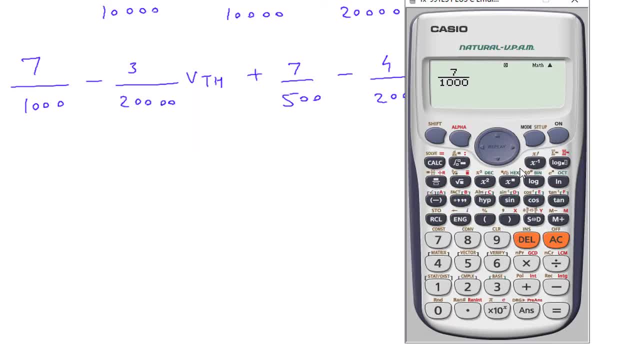 Then plus 7 by 1000.. 7 by 1000.. 7 by 500.. So this will be 0.021.. 0.021. 0.021. 0.021. 0.021.. 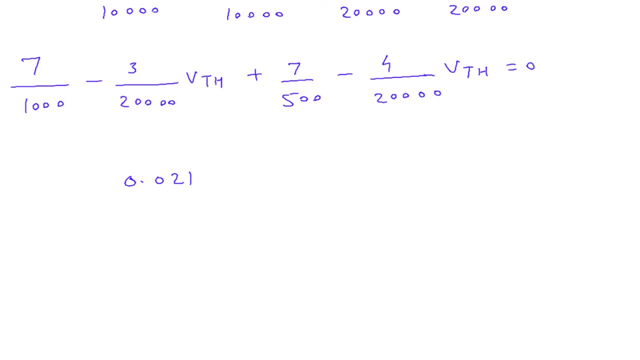 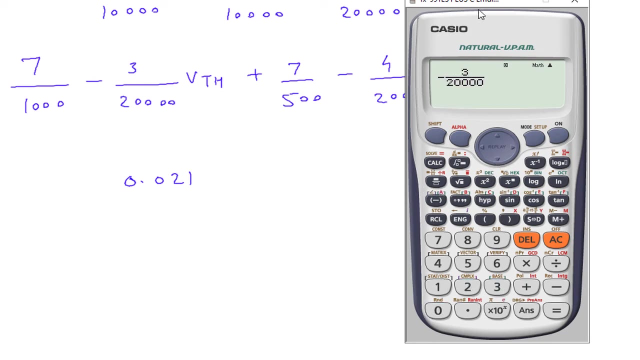 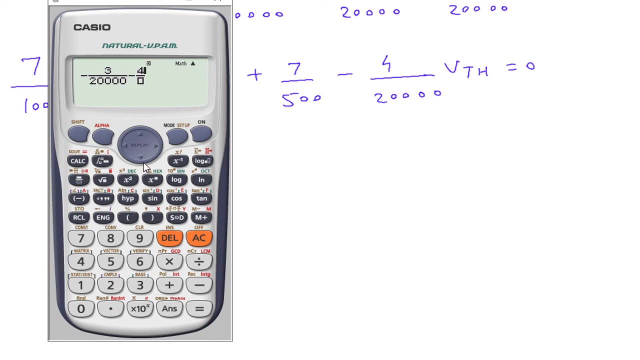 Then this will be: Minus 3 by Minus 3 by Minus 3 by 20,000.. 20,000.. Then minus 4 by Minus 4 by 20,000.. 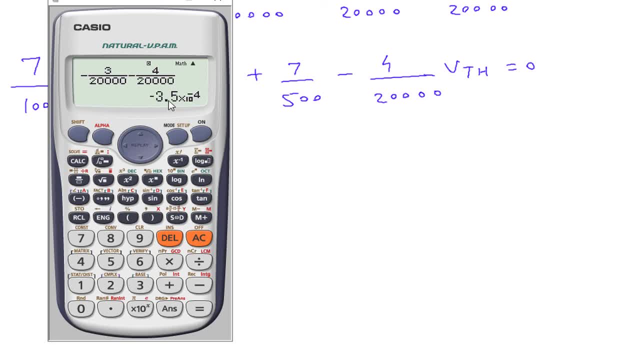 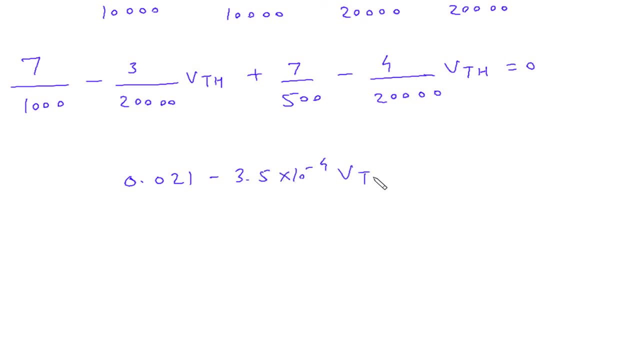 20,000.. So this will be Minus 3.5.. Minus 3.5 into 10, raised to 4 by VTH, is equal to 0.. Now this will be 0W. Now this will be. 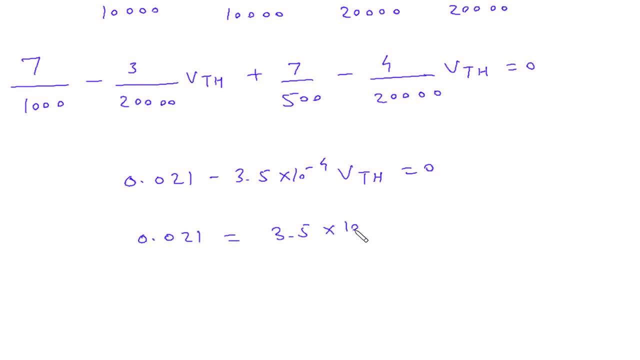 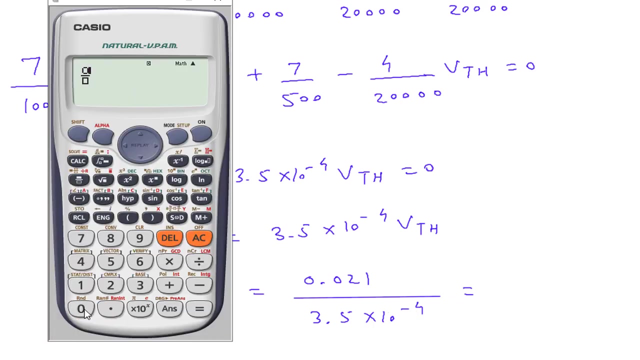 0.021 is equal to 3.5 into 10 raised to the power minus 4. VTH From this, VTH is equal to: VTH is equal to 0.021 divided by 3.5 into 10 raised to the power minus 4. so this will be 0.021 divided. 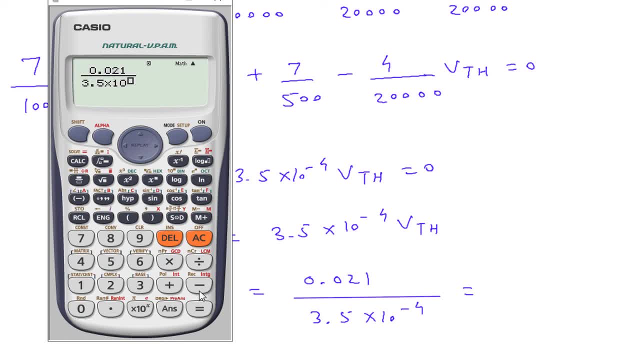 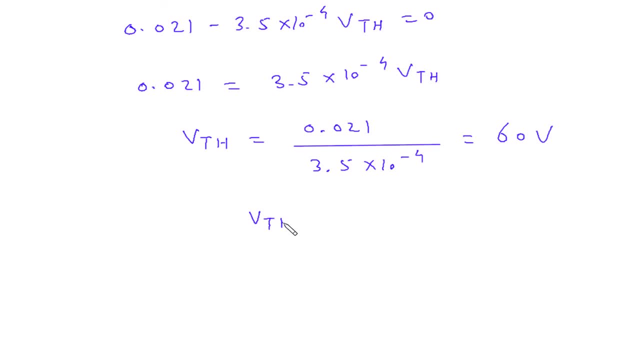 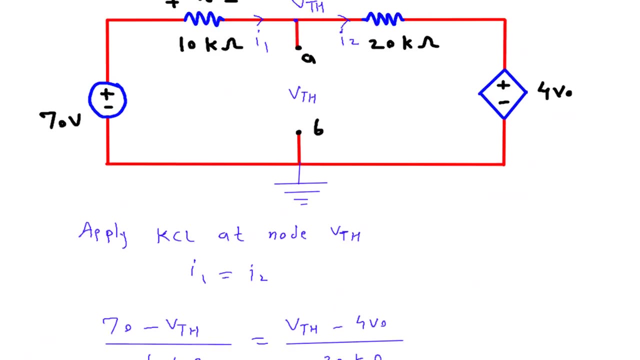 by 3.5 into 10, raised to the power minus 4, so this is 60 volt. therefore, Vth is equal to 60 volt and Rth is equal to. Rth is equal to 2.857 kilo ohm. what we have to find we